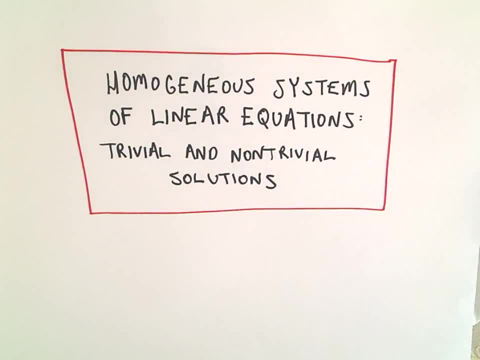 Alright, in this video I want to start looking at the notion of homogenous systems of linear equations and we're going to talk about what are called trivial and non-trivial solutions. So in this video we're going to look at a couple examples that have trivial solutions and then in a separate video we'll do an example that has non-trivial solutions, just because the row reduction can take a little bit of time. 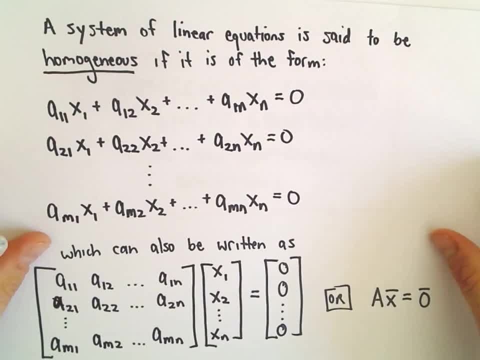 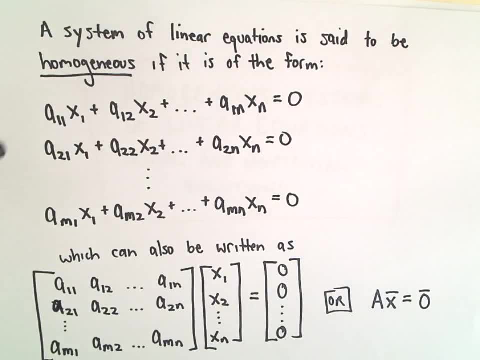 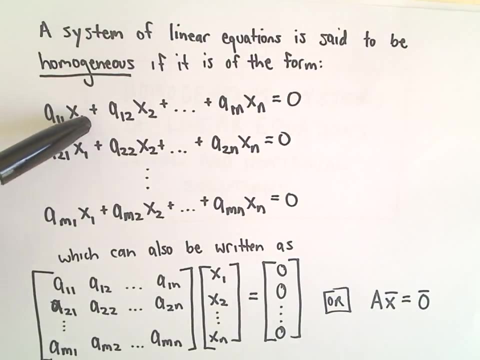 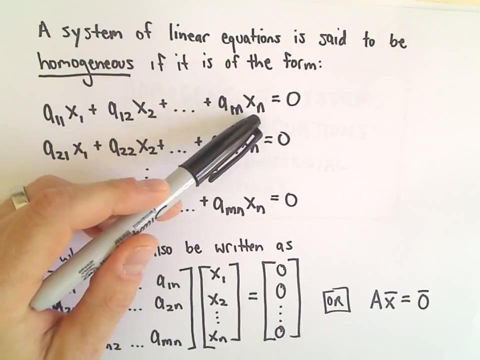 Okay. so I guess let's just start off with a little definition here. So we say a system of linear equations is homogenous if it's of the form. so we've got some coefficients: the a sub 1, 1 times the variable x sub 1,, plus a sub 1,, 2 times the variable x sub 2, plus dot, dot, dot. a sub 1, n times the variable x sub n equals 0.. 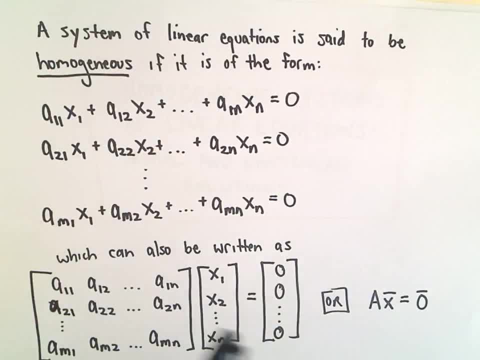 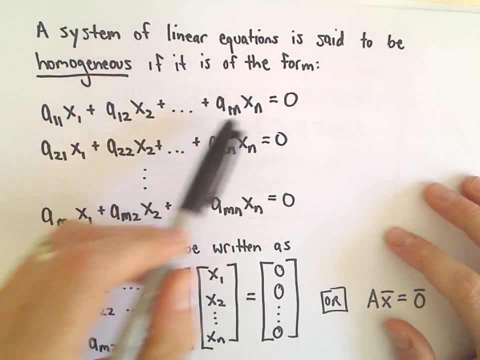 And you can. you know, this is kind of our first row, Okay, And then our second row, Okay, And then our second row and then down to the mth row. So basically we just have a bunch of linear equations, variables being multiplied by coefficients- real number coefficients- and again it's homogenous if all the coefficients on the right side are 0.. Okay, so that's what we're looking for. are the 0s on the right side? 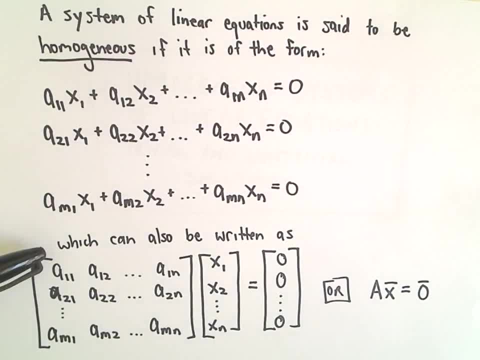 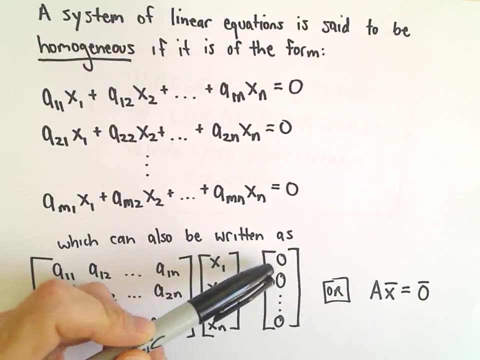 We can also write this as a little matrix equation and we can write that by just taking the coefficients putting those in one matrix. We can also write that by just taking the coefficients putting those in one matrix, multiplying that by the vector x sub 1, x sub 2, down to x sub n, so we have our variables and then we just set that equal to a bunch of 0s. 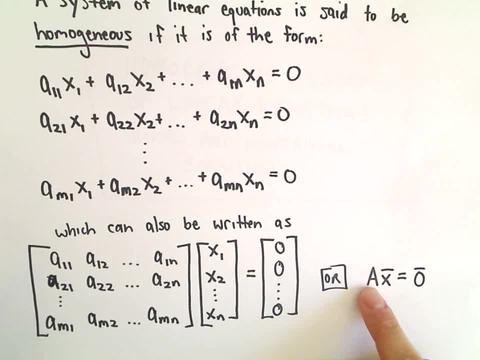 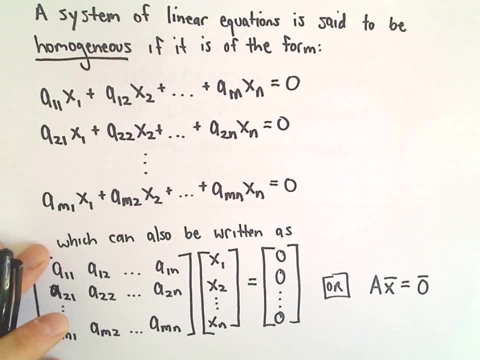 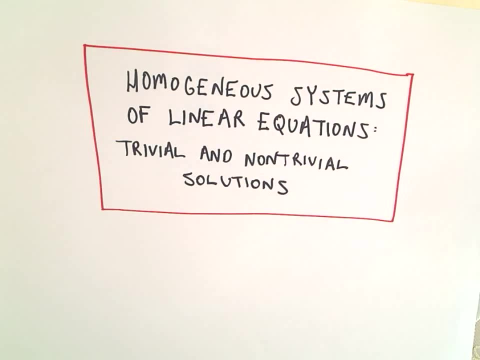 So again, more shorthand, we can write this as the matrix. this would be our matrix A times our vector x, and we want that to equal the 0 vector. So that's the definition of a homogenous system. So now homogenous systems can have again what are called trivial orders. 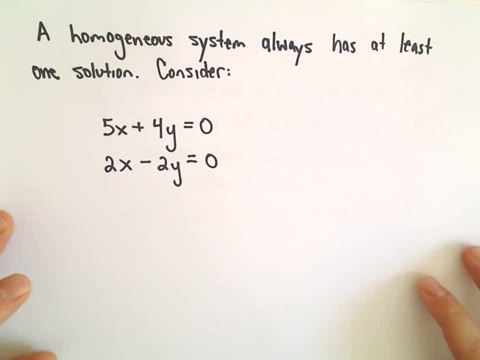 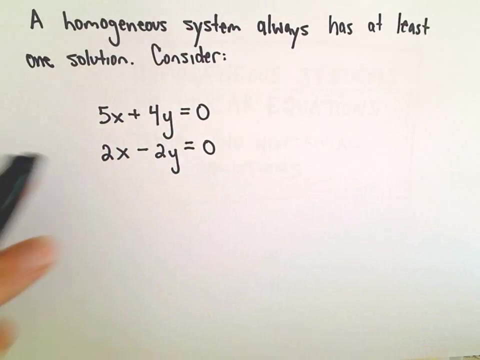 They're called non-trivial solutions, and one thing that happens is a homogenous system always has at least one solution, So the one solution is going to be the trivial solution. so let's look at this system: 5x plus 4y equals 0,. 2x minus 2y equals 0.. 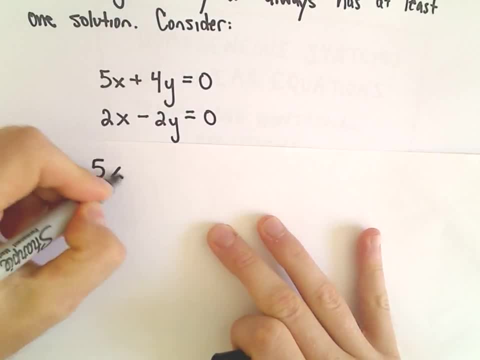 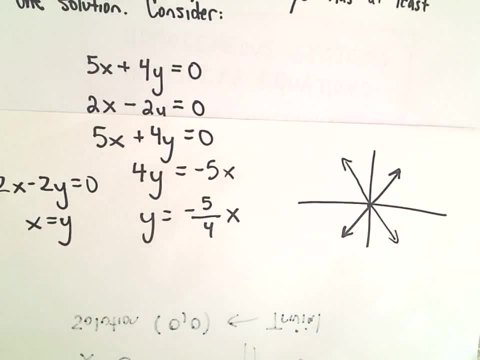 So notice, if we multiply the second equation by 2, we'll get 4x minus 2y equals 0. I think that's something that's important as well. You know certainly a little harder to graph the larger ones, But would like to tie in some geometry to some of these. 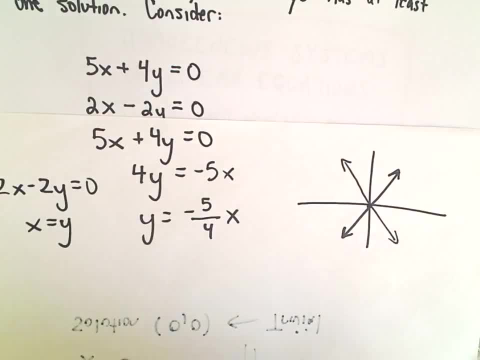 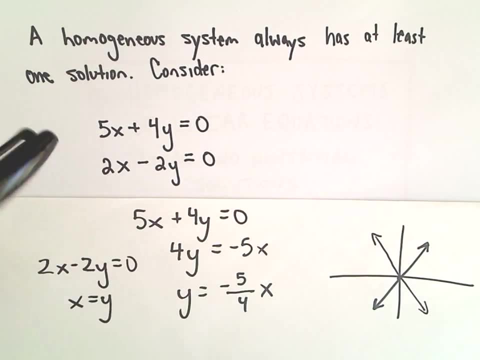 I think it's just another way to think about them. So again, just to remind you of that, No big deal, OK. So again, a homogenous system always has at least one solution, In this case the trivial solution 0, 0.. 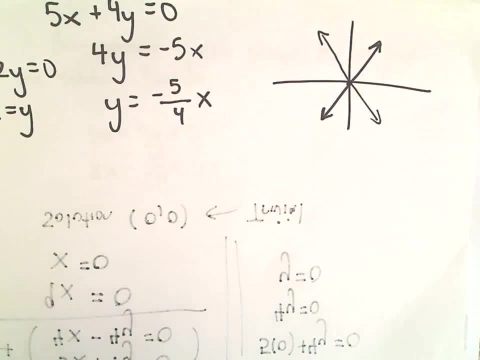 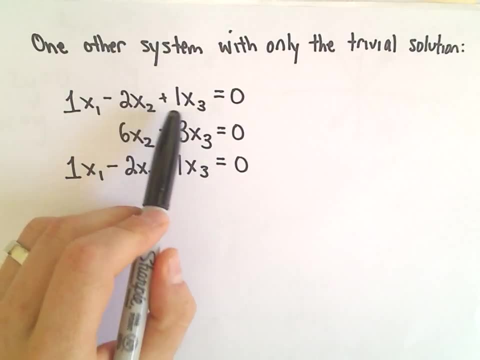 Nothing, nothing else other than that. Let's look at maybe one more example here that only has the trivial solution 3Аy. So we have 1x sub 1 minus 2x sub 2 plus x sub 3, equals 0,. 6x sub 2 minus 3x sub 3 equals 0,. 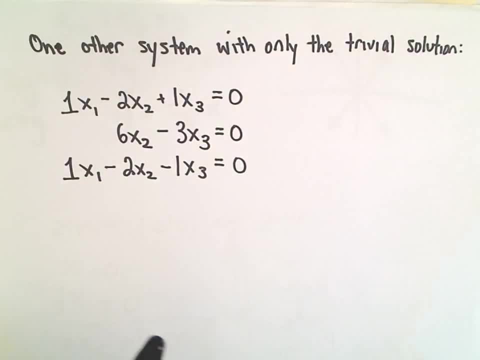 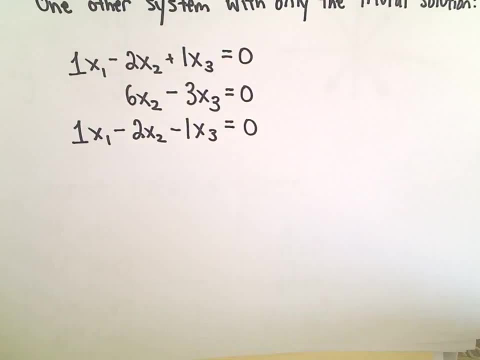 and then 1x sub 1 minus 2x sub 2 minus x sub 3 equals 0.. Again, let's just show that this only has the trivial solution. So again, we could do our elimination by addition or substitution, or however you want to do it. 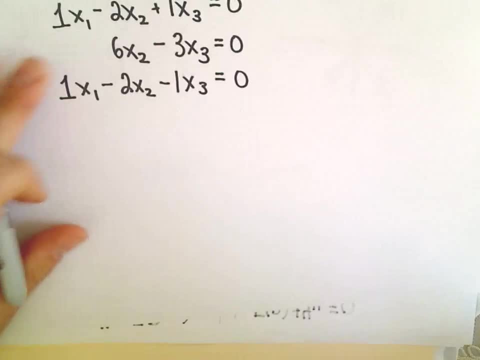 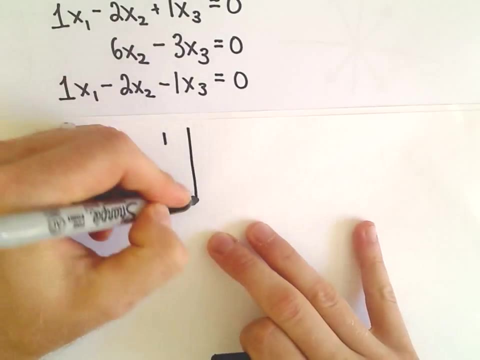 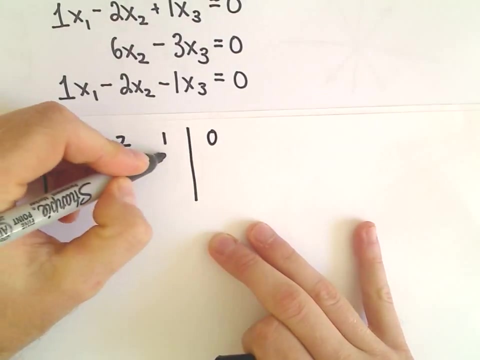 I'm certainly going to start using some row reduction here, So I'm going to write my matrix with my coefficients. So we have 1, negative, 2, positive, 1, 0. on the right side We have 0x sub 1, so we have positive 6x sub 2 minus 3 equals 0.. 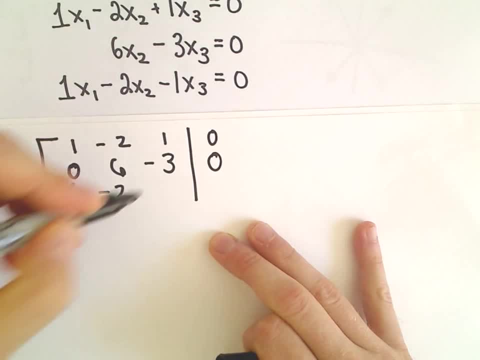 And then we've got 1x sub 1 minus 2x sub 2 minus 1x sub 3, and then we have 0 again on the right side. So I'm going to do some row reduction here. So the first thing: 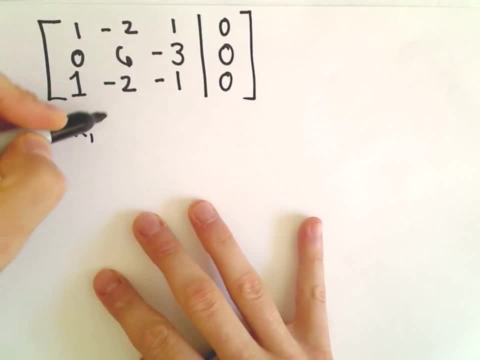 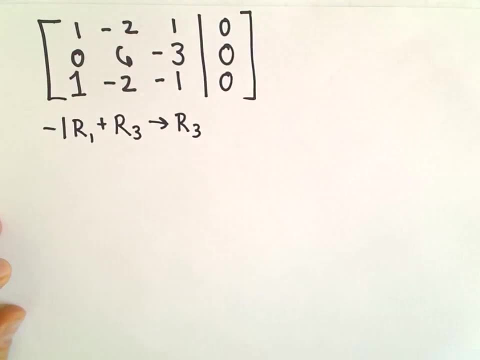 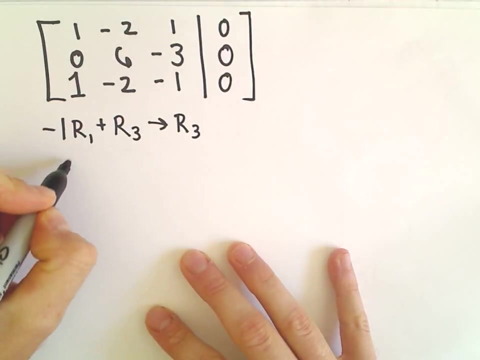 What I'm going to do is I'm going to take negative 1 times the first row, add that to my third row and that's going to produce my new third row. I think one other thing I'm going to do here at the same time is I'm going to take my second row and I think I'm going to just divide it by 3.. 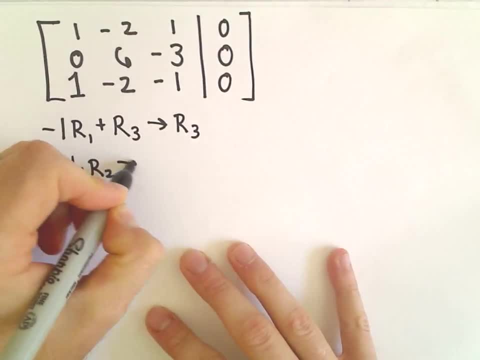 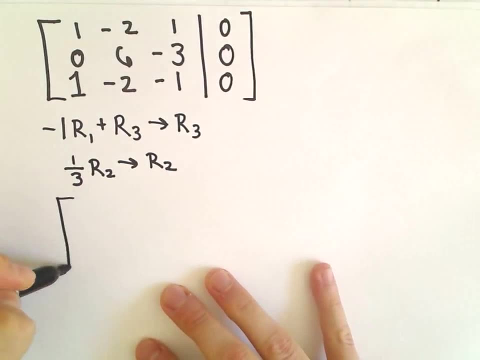 So I'm going to take 1 third row 2 and that's going to give me my new row 2, just because I see that everything's divisible by 3, just to make the numbers a little bit easier. So not really doing anything with the first row, so let me just jot those right-back down. 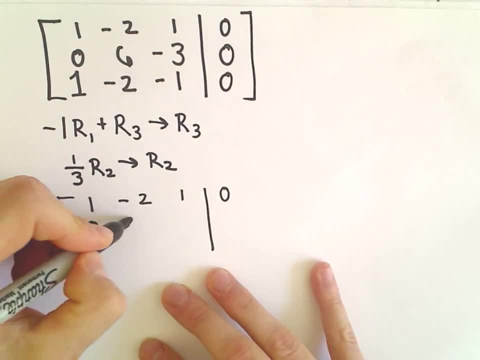 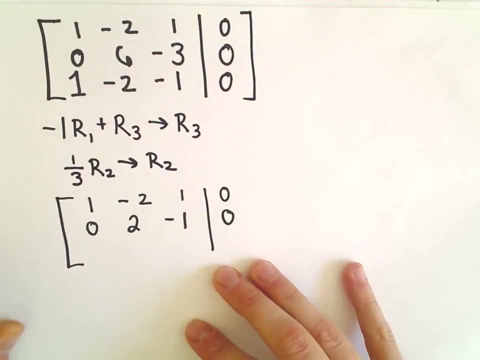 Well, if I take the second row and divide it by 3, I'll have 0.. 6 divided by 3 is 2.. Negative 3 divided by 3 is negative 1, and then we have another 0.. So now, if we do our first little step here, so if I take negative 1 times 1, that'll be negative. 1 plus 1, is 0.. 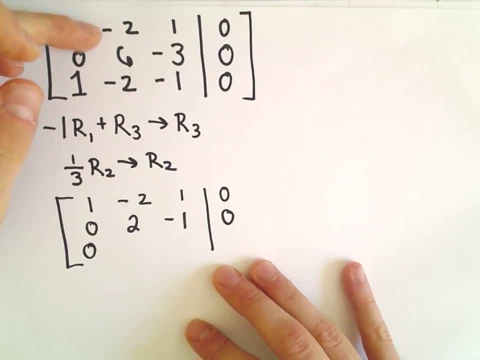 Let's see: Negative 1 times negative 2 is positive 2, Plus negative 2, again will give us 0.. Negative 1 times 1 is negative 1.. Plus negative 1, that's going to give us negative 2.. 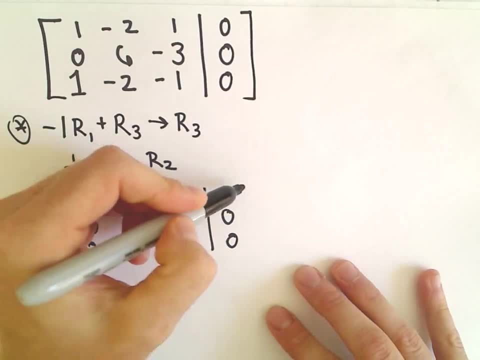 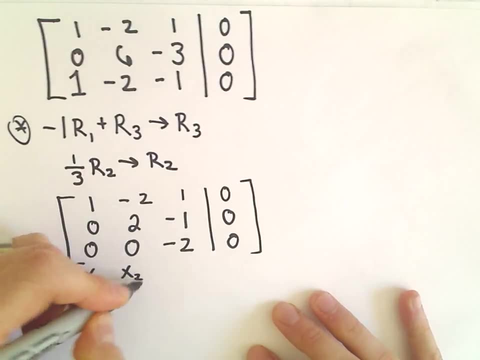 And again the 0s will all stay simply 0.. Well, let's think about what this really says now. So again we had our variables x sub 1, x sub 2, and x sub 3.. So the thing that's kind of cluing me into this trivial solution is this last row that I'm looking at here. 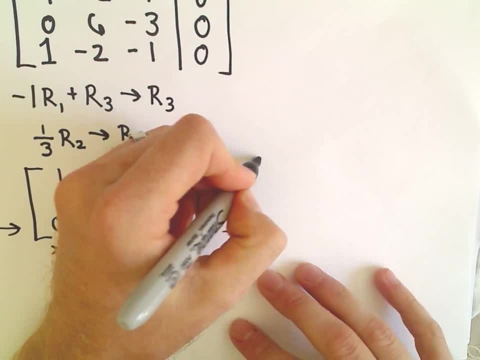 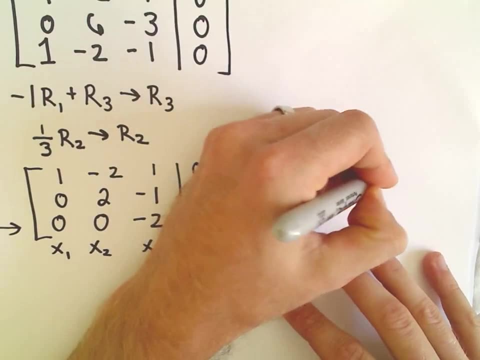 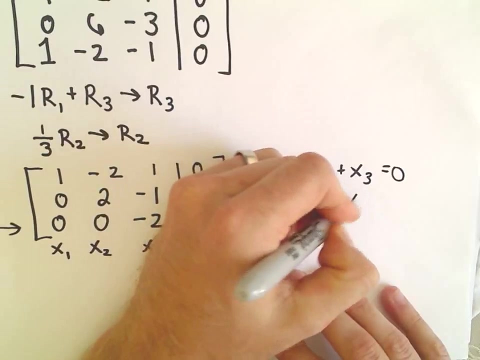 So notice. we could rewrite this as a system of equations. The first one simply says that 1x sub 1 minus 2x sub 2 plus x sub 3 equals 0. So basically what we started with. The second row says that 2x sub 2 minus 1x sub 3 equals 0..